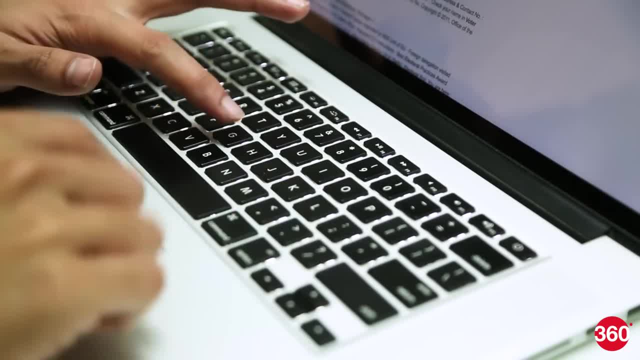 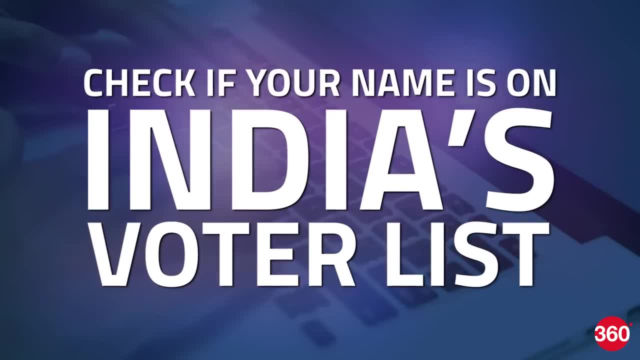 That's why it's very important to check if your name is on the voter list well in advance of the elections. Follow these steps. to check if your name is on electoral rolls in India: Go to the National Voter Services Portal's electoral search page. Here you can. 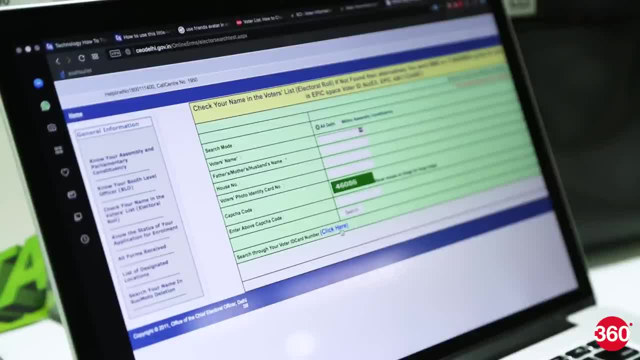 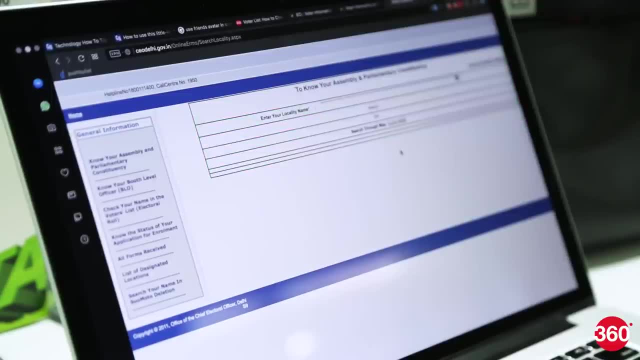 search for your name on the voter list by two methods: manually entering all of your details or simply by entering your electoral photo ID card number. The EPIC number is mentioned in bold letters on your voter identity card. If you have an EPIC number, go through these steps to check if your name is on the voter list. 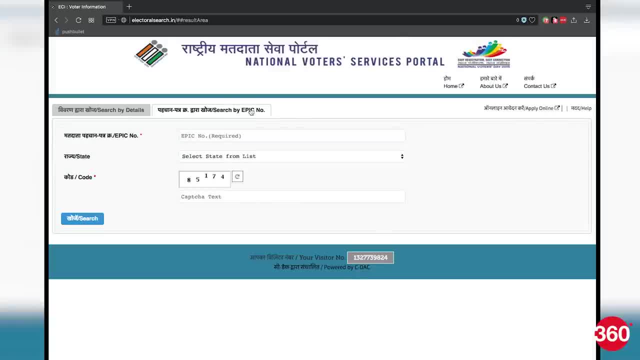 Visit the electoral search page. click or tap on the search by EPIC number. enter your EPIC number, select a state from the drop-down menu and key in the code you see on the image. Then click or tap search. If your name is on electoral rolls, you will be able to see it. 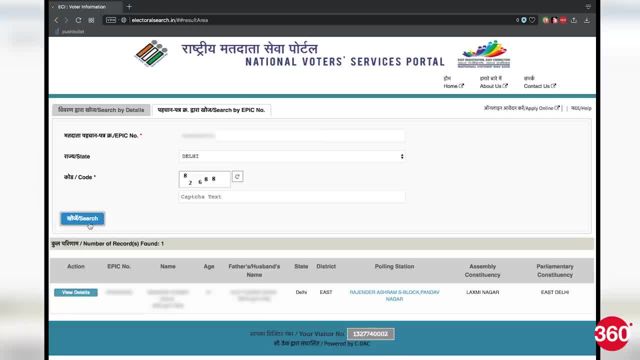 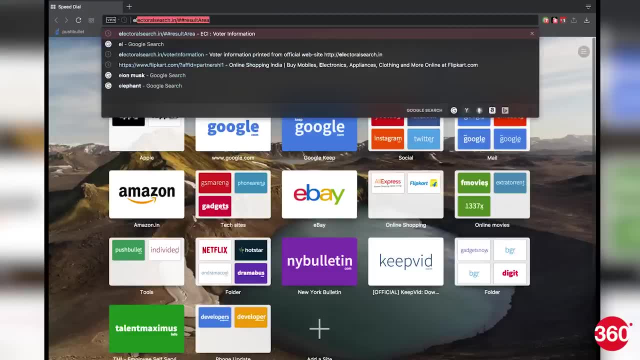 below the search button. If nothing shows up, there is a good chance that your name is not on the voter list. In case you don't have your voter identity card with you and thereby you don't have your EPIC number, these steps should help you check if your name is on the voter list. 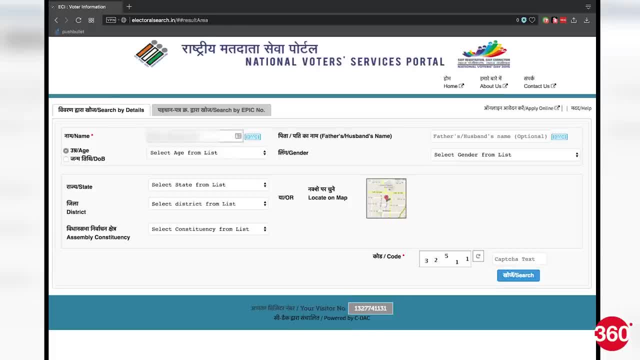 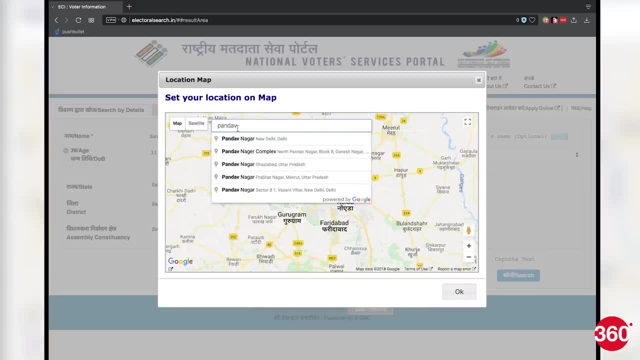 Visit the electoral search page. click or tap on search by details. Key in all the details, including your name, gender, age, assembly, constituency, etc. as described on the page. Then you enter the code on the captcha image and finally click or tap on search. 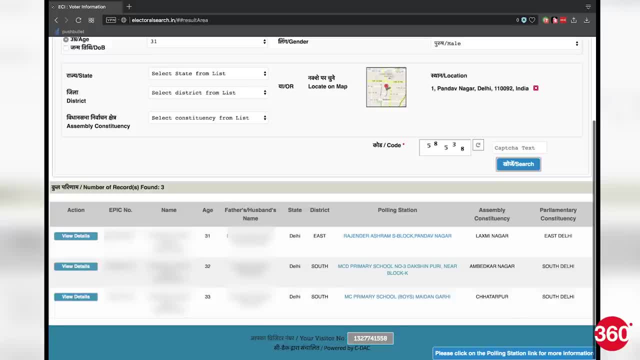 If you see a result in the area below the search button, that means your name is on the voter list. If not, then it's probably not there. We know several people whose names have been misspelled on their voter ID cards and there is a chance that the search by details. 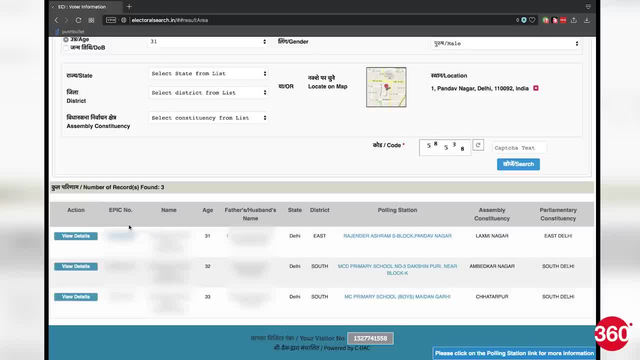 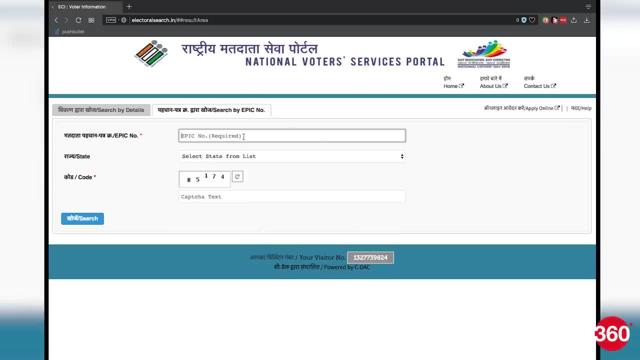 method isn't yielding the desired results because the spelling of the name doesn't match that on the election commission's database. That is why we suggest that you look for your name on electoral rolls via the EPIC number, as it's far less likely to return a false result. 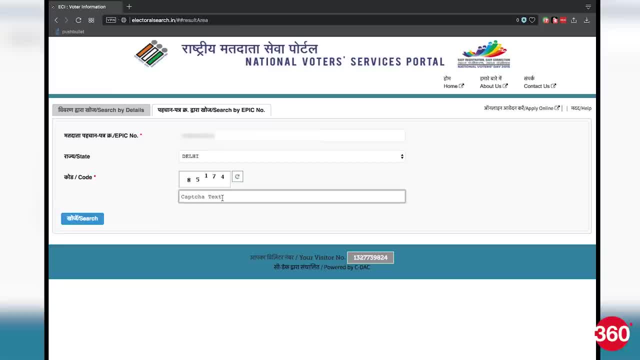 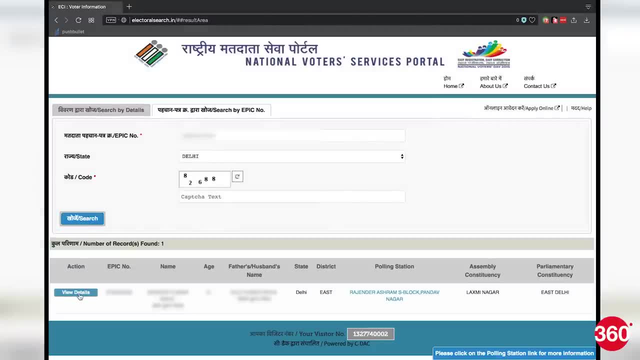 If you liked this video, don't forget to share it with your friends. You can also follow Gadgets360.com for more news, reviews and features. Thank you for watching and see you in the next video.